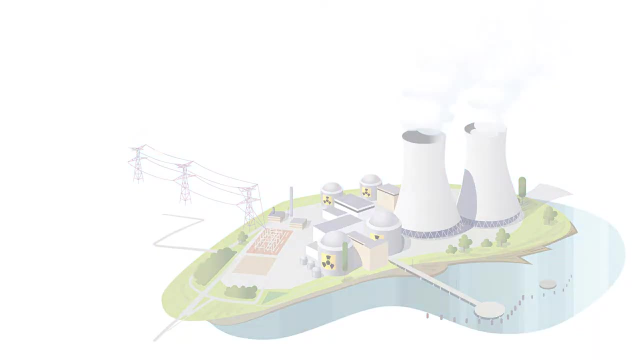 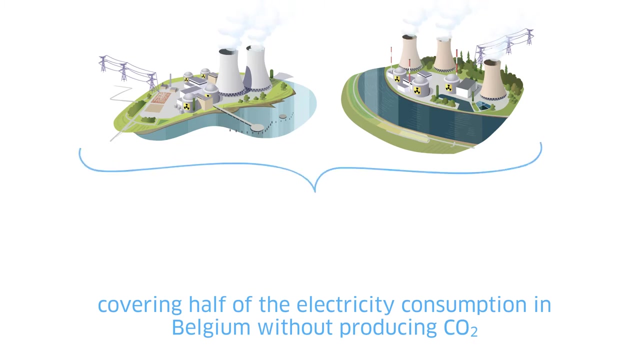 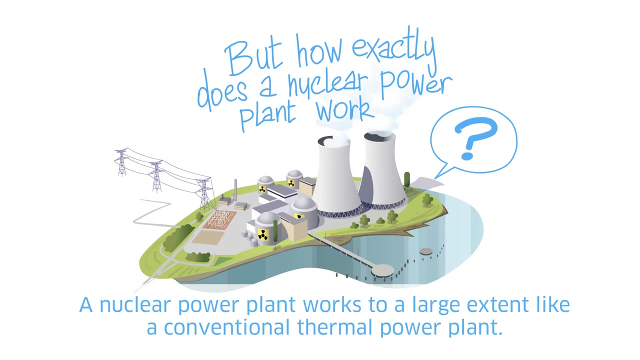 Electrabel has seven nuclear power plants, four in Doules and three in Tiange, covering half of the electricity consumption in Belgium without producing CO2.. But how exactly does a nuclear power plant work? A nuclear power plant works to a large extent like a conventional thermal power plant. 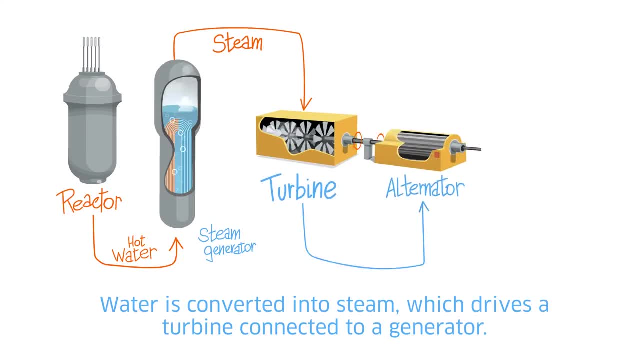 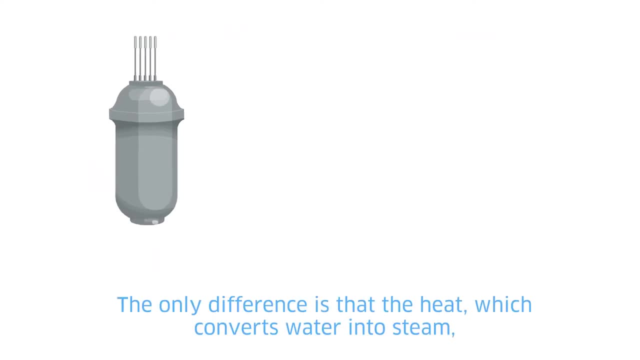 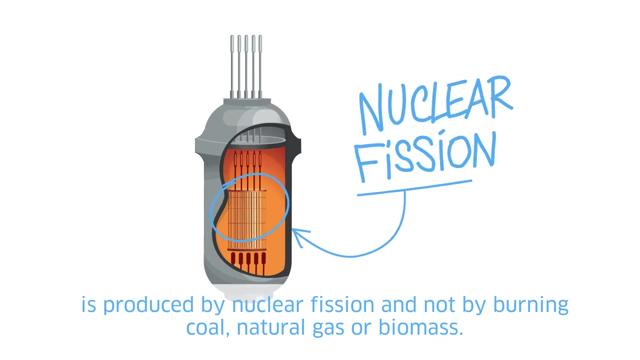 Water is converted into steam, which drives a turbine connected to a generator. This generator converts the mechanical energy into electrical energy. The only difference is that the heat which converts water into steam is produced by nuclear fission and not by burning coal, natural gas or biomass. 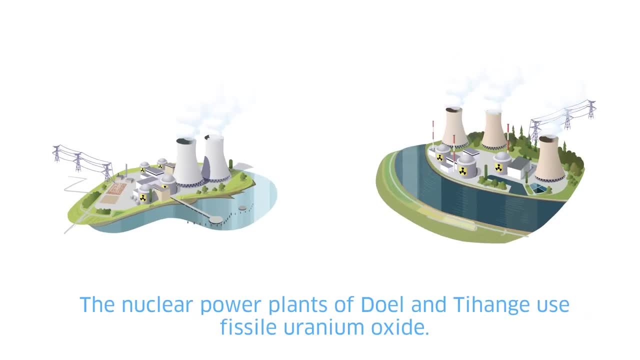 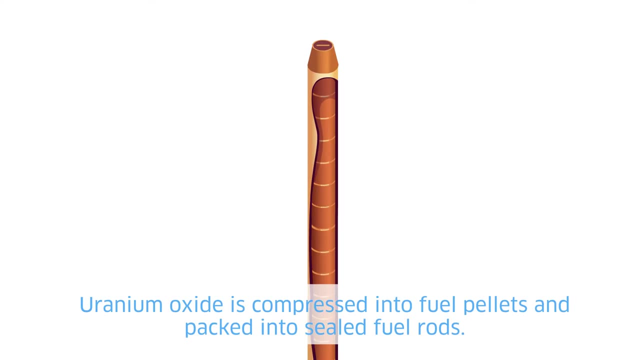 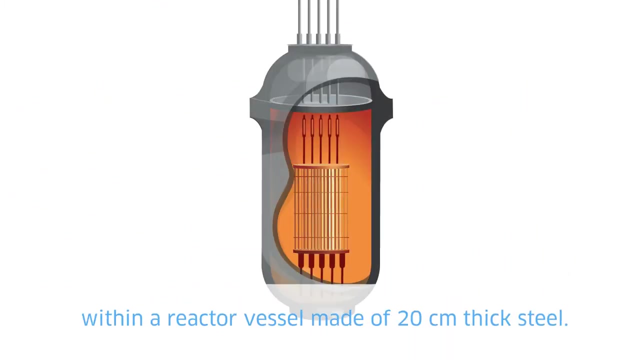 The nuclear power plants of Doules and Tiange use fissile uranium oxide. Uranium oxide is compressed into fuel pellets and packed into sealed fuel rods. Multiple rods in turn form fuel elements which are immersed in water. The reactor vessel is made of 20 cm thick steel. 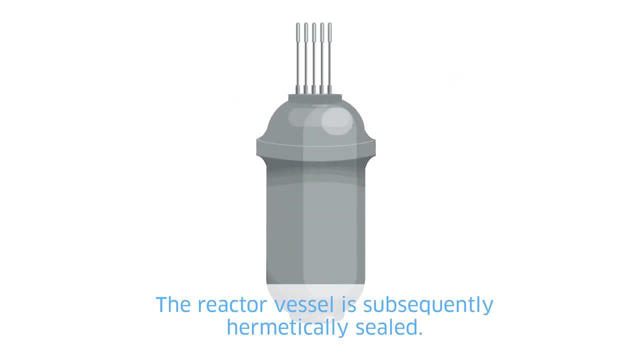 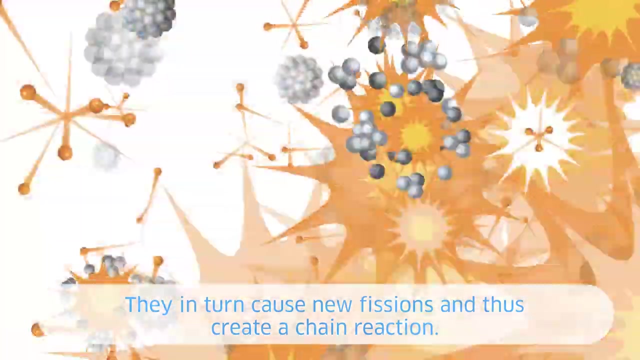 The reactor vessel is subsequently hermetically sealed. The fission of the uranium can now begin by bombarding it with neutrons. In each fission, two or three neutrons are released. They in turn cause new fissions and thus create a chain reaction. 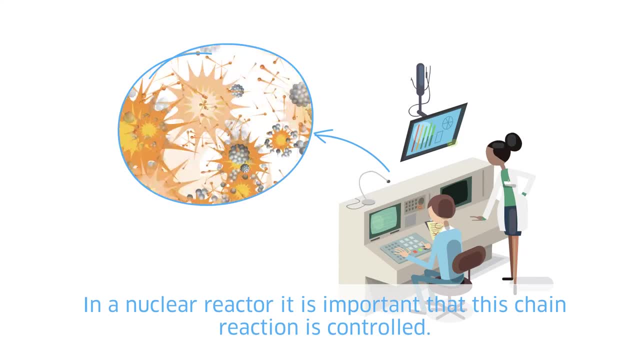 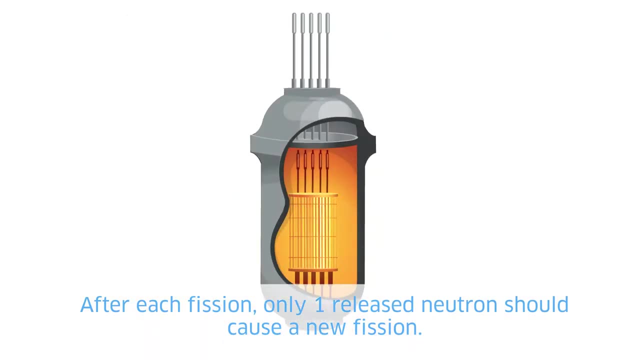 In a nuclear reactor. it is important that this chain reaction is controlled. After each fission, only one fission is released. One released neutron should cause a new fission. Boric acid in the water of the reactor vessel and lowered control rods absorb the oversupply of neutrons. 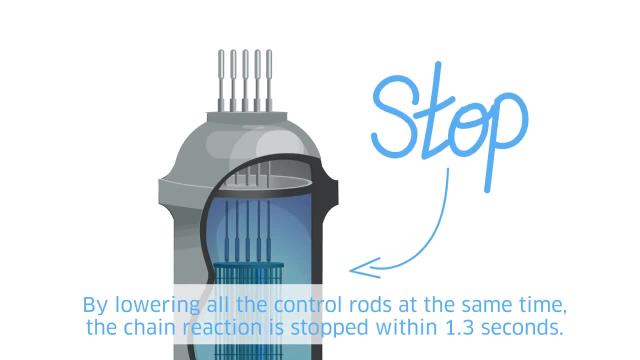 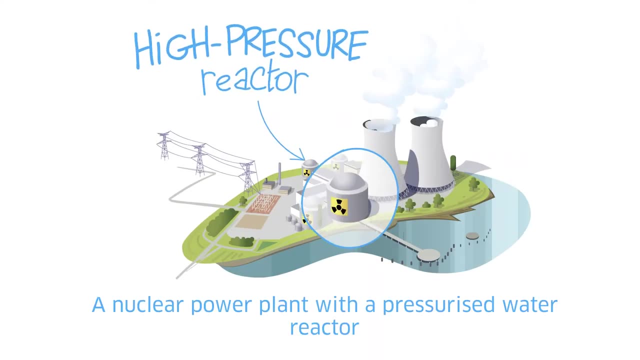 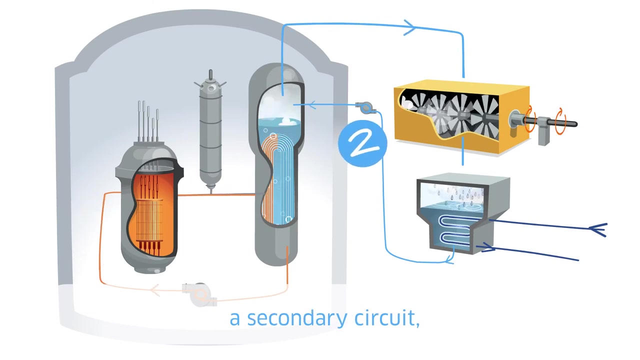 By lowering all the control rods at the same time, the chain reaction is stopped within 1.3 seconds. A nuclear power plant with a pressurized water reactor, such as Doules and Tiange, has three completely separated water circuits: A primary circuit, a secondary circuit, a tertiary circuit. 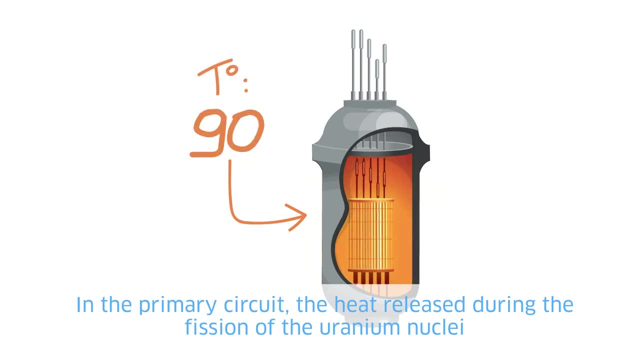 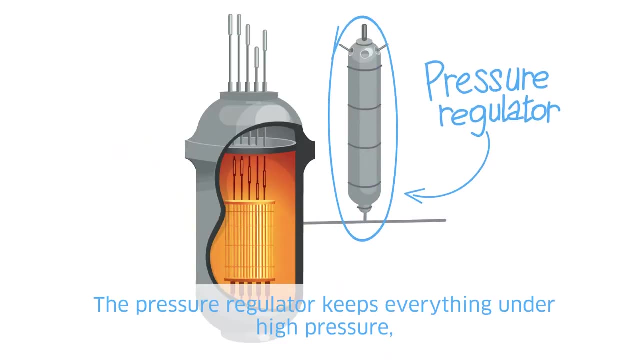 In a primary circuit. the heat released during the fission of the uranium nuclei heats up the water in the reactor vessel to the temperature of 320°C. The pressure regulator keeps everything under high pressure, so the water does not boil or form steam.